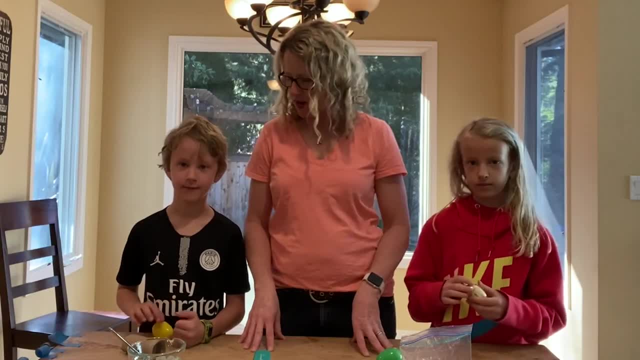 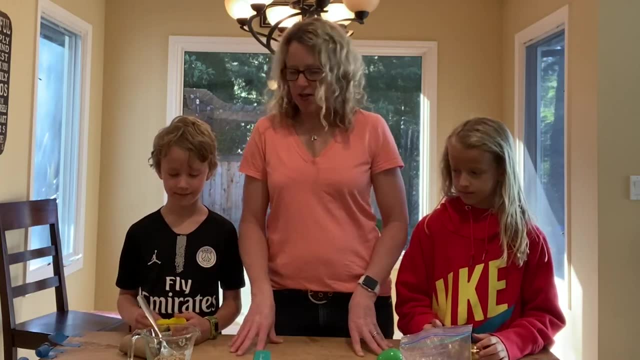 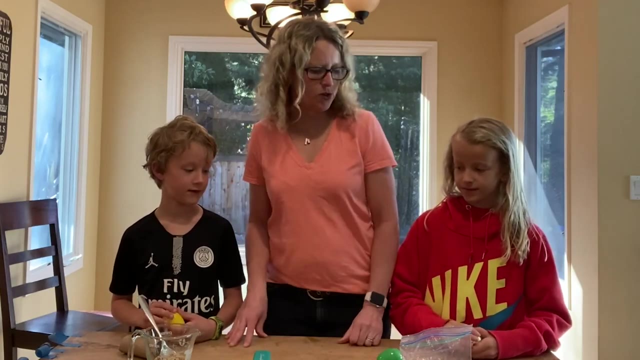 those. grab those. So first we'll start with those. Ryder and Cora. So Ryder's got some dry garbanzo beans and that's what he's using to make his shaker, And Cora found some beads to make her shaker. So why don't you go ahead and scoop your beans out of the shaker And 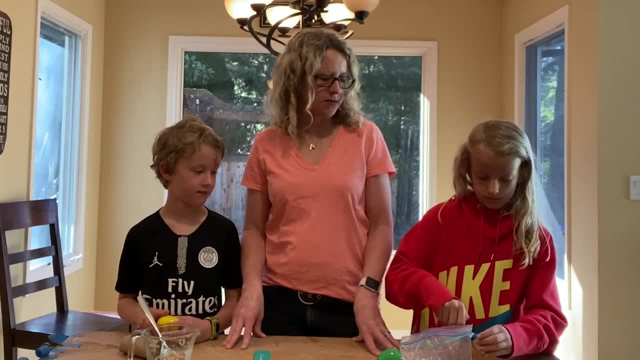 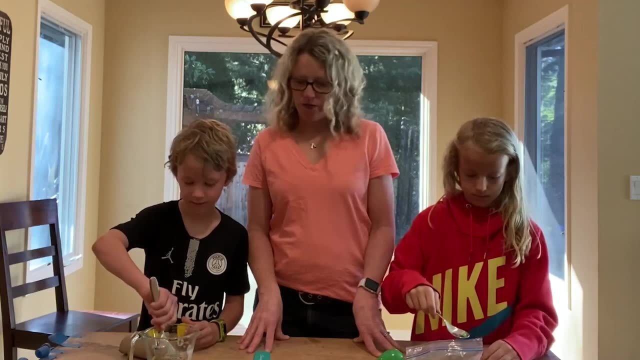 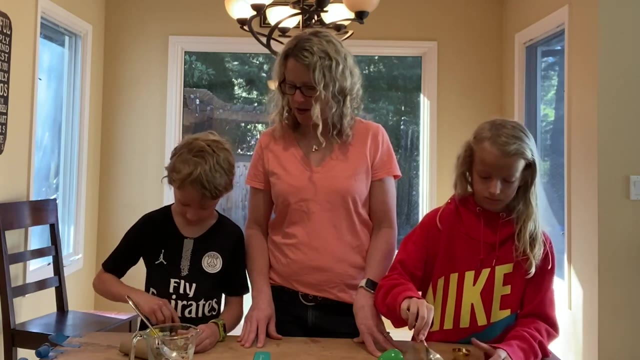 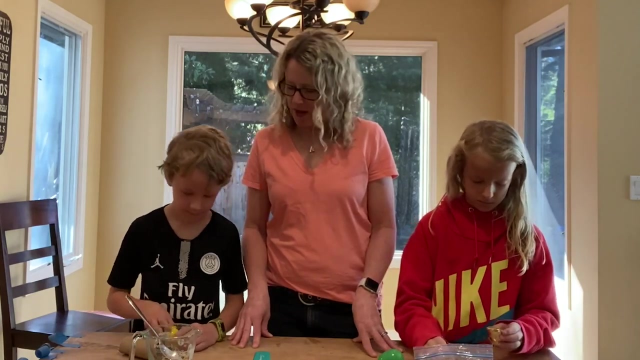 you're going to scoop your beans and your beads into your shakers, So use your spoon and go ahead and fill your eggs. You do half at a time- And then, if you're doing these with kids that are a little bit younger, you definitely want to secure these eggs and shakers. 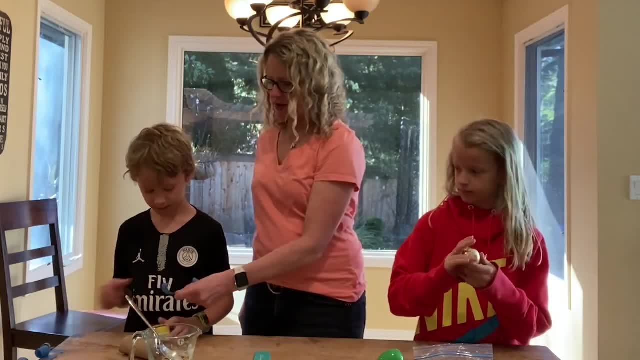 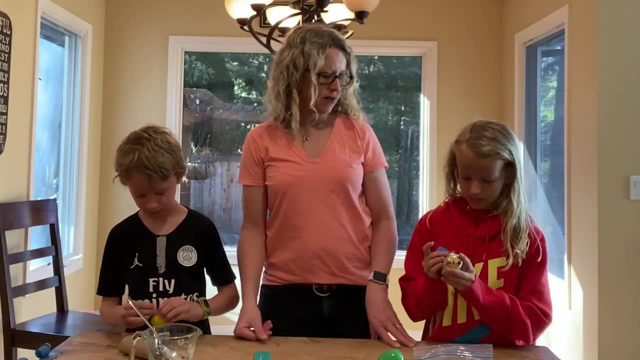 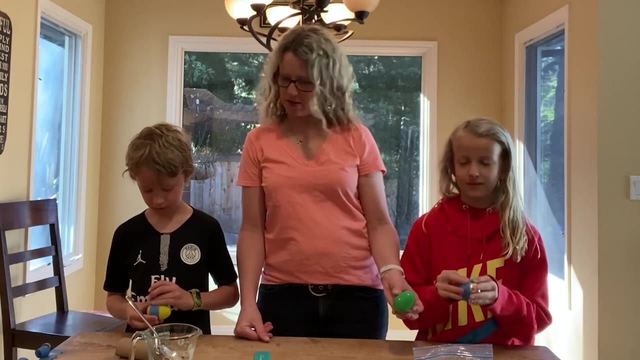 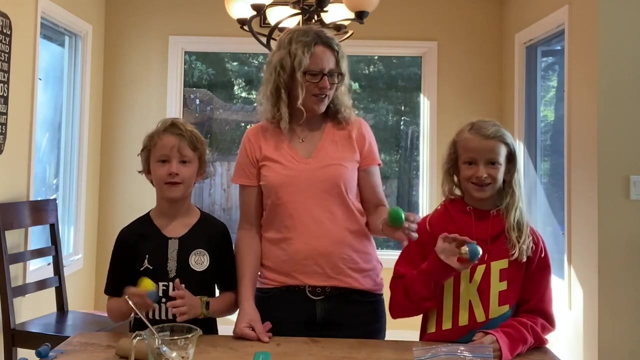 with tape. So grab a piece of tape and go around the seam so that it's nice and tight, Nice and secure And nothing will fall out. There you go. Cora already made one, So she's got two egg shakers. All right, let's hear them shake. That's the egg shaker. Okay Now. 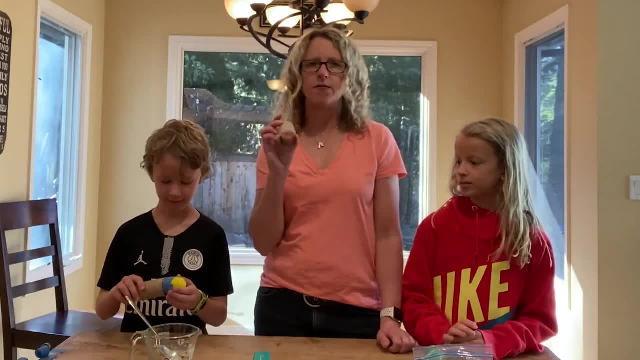 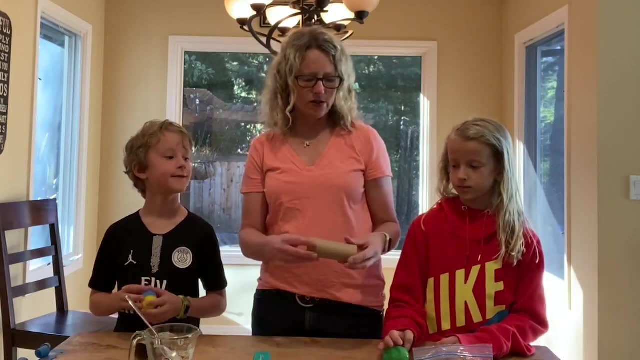 the other thing we grabbed was just empty toilet paper rolls made of cardboard. So there were two of them. So we're going to go ahead and scoop those out of the shaker, And then we're going to take our bowl and cut off these ends here so we don't have any more. 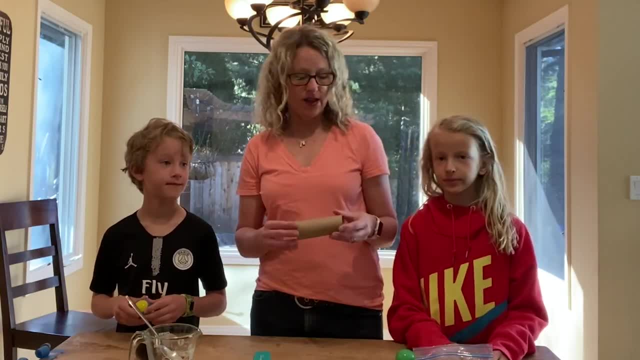 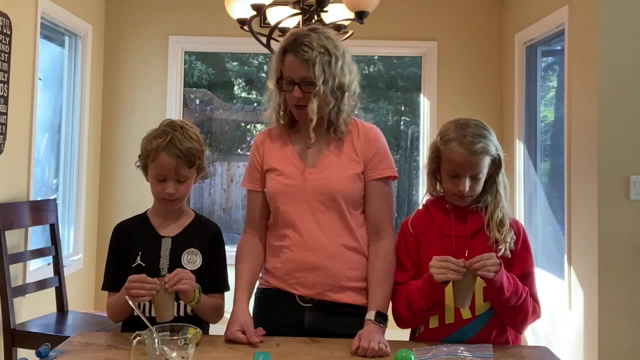 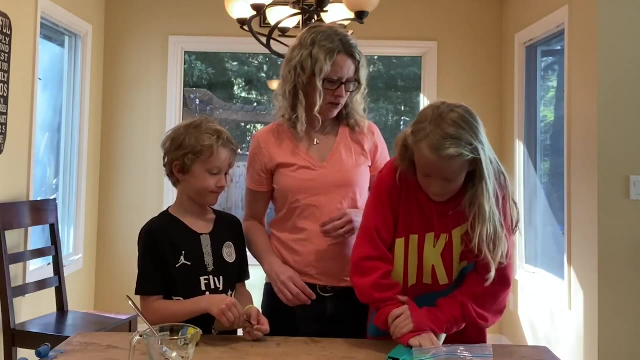 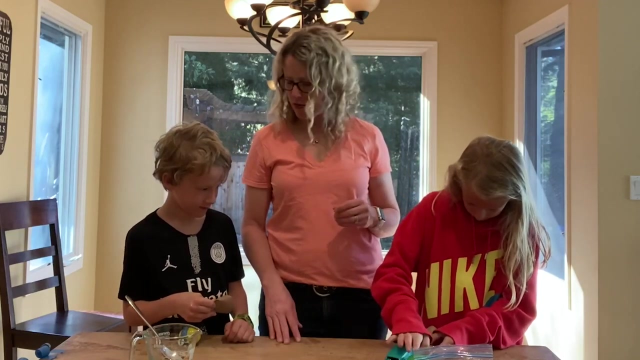 ice in them. So you get just a small Realm милли bag. but then the ground is but awesome. Let's see how we're going to wrap this around. the supposedly No from now. Here we go��. So now we're going to tie our end, and then we're going to sew the end, So we're just 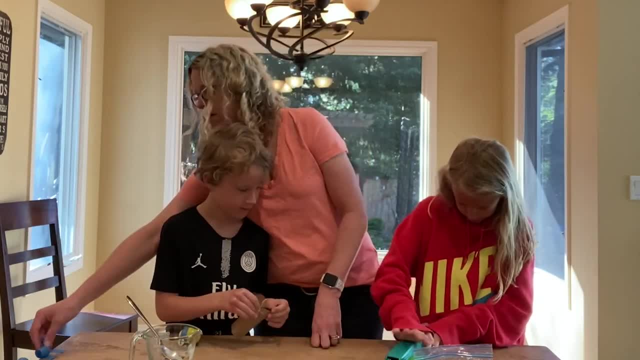 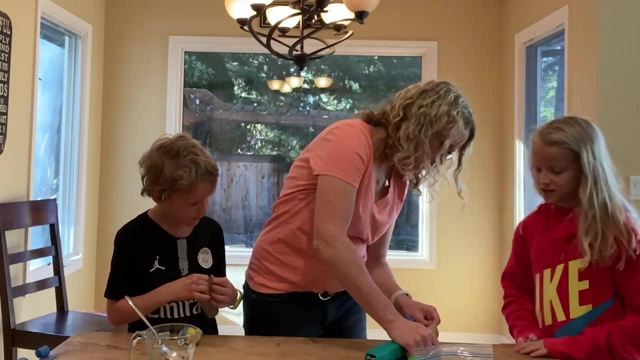 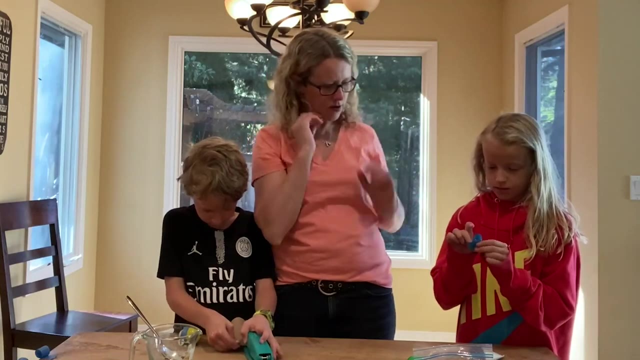 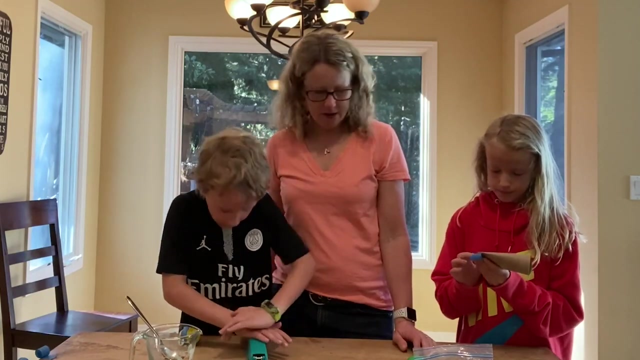 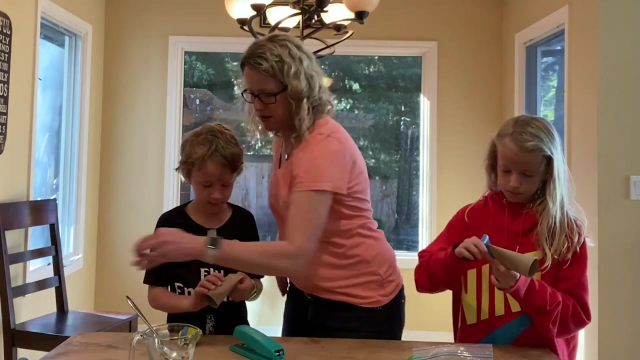 and then you'll want to secure it with some tape. you need a little help there. all right, all right, there you go. now secure that one end with tape, just to make sure nothing comes out. you can use masking tape or packing tape. this is just some blue painters tape that I had laying around. let's do one more to.